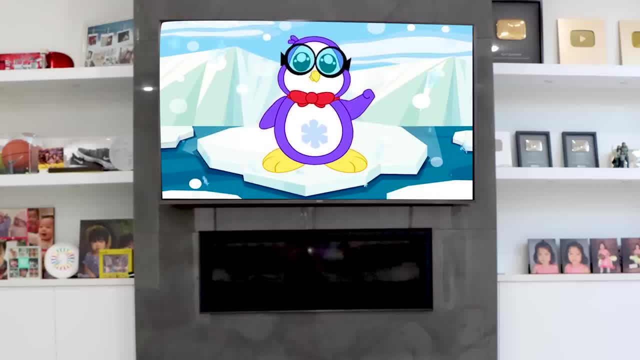 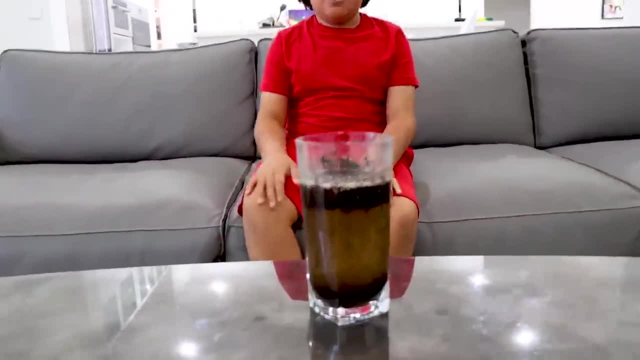 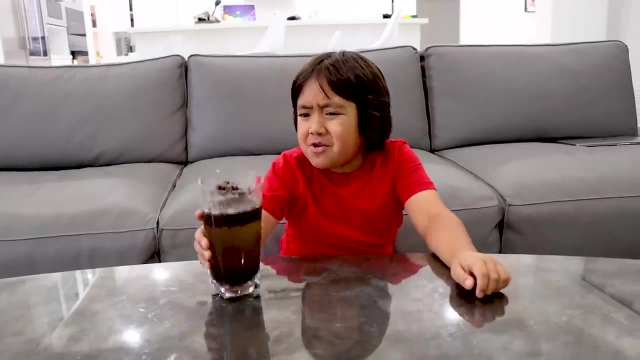 Whoa, Hey, Ryan, Who's that? Is that you Peck, Peck. what is this? Oops, sorry, Ryan, I left a glass of dirty water there on accident. Ivo, you cannot drink this. This is dirty. Welcome to Ryan's World. 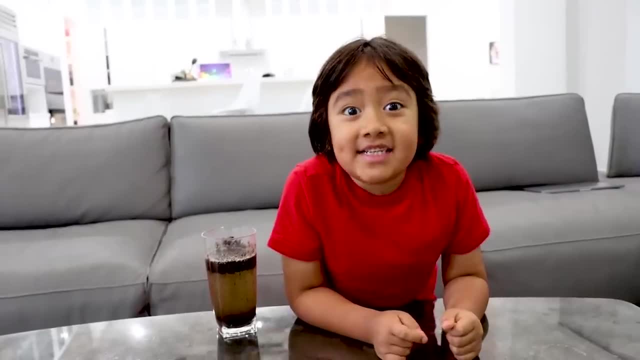 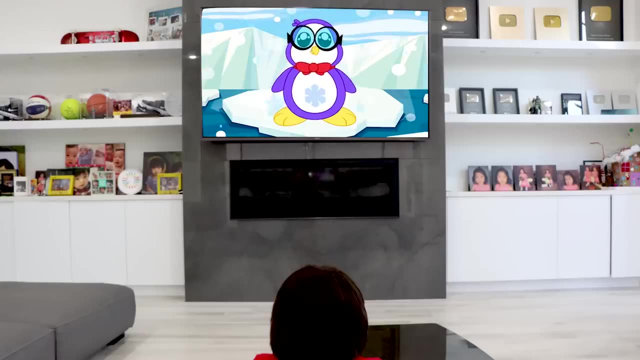 Peck. I have an idea: Maybe there's a way to filter out all the dirty stuff. Send it to the lab, Ryan, and I'll find a way to get the dirt out. I'm sending this water to you. Peck Teleportation device. 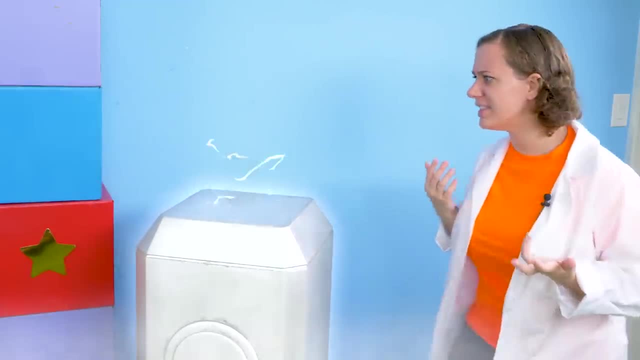 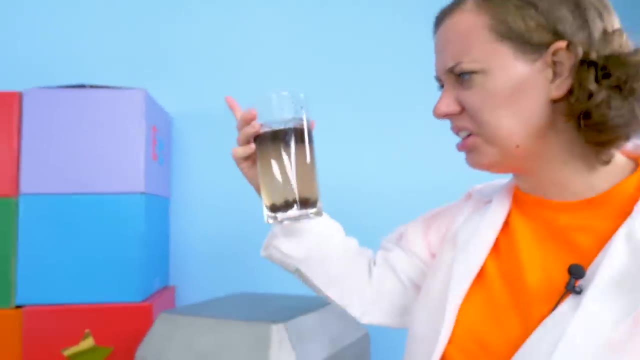 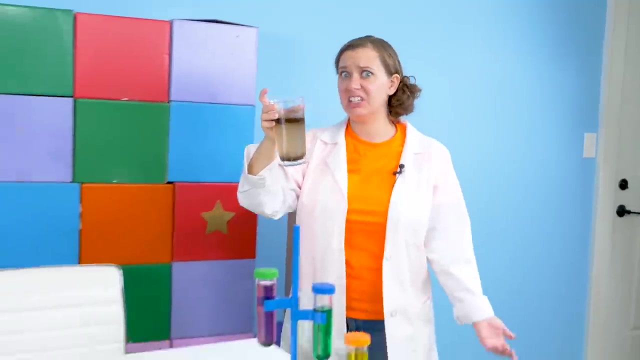 It looks like Ryan is sending us another science experiment. I wonder what this one could be. Hmm, Wait a second. Is that water? It's really dirty water. We can't do anything with this. We really need to clean this water up. I know just who to call for help. We need Peck. 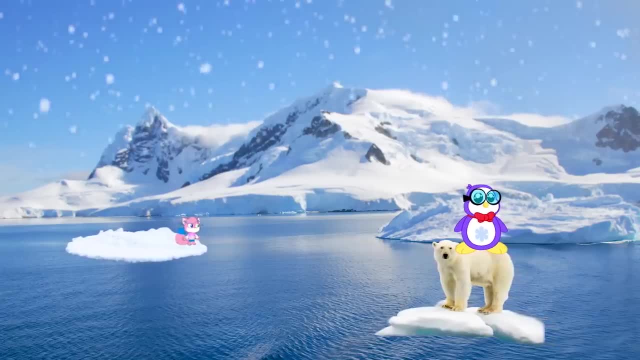 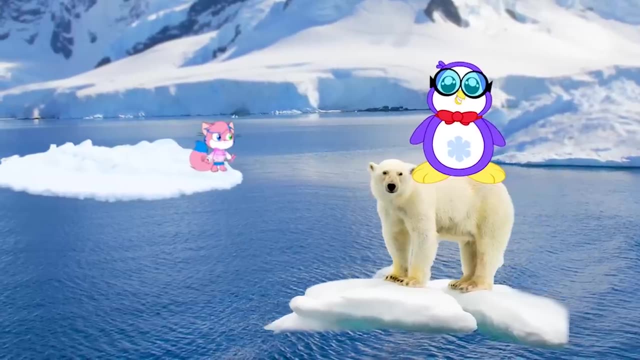 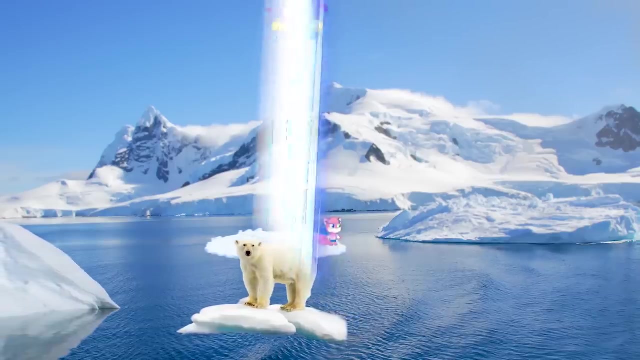 Peck, Peck. Get this way for another 8,000 miles and you should make it to the North Pole. Huh, Looks like I'm needed in the lab Later. buddy, Woo-hoo. What's today's science experiment? 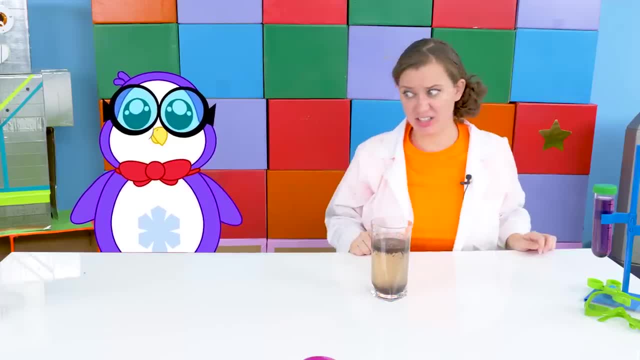 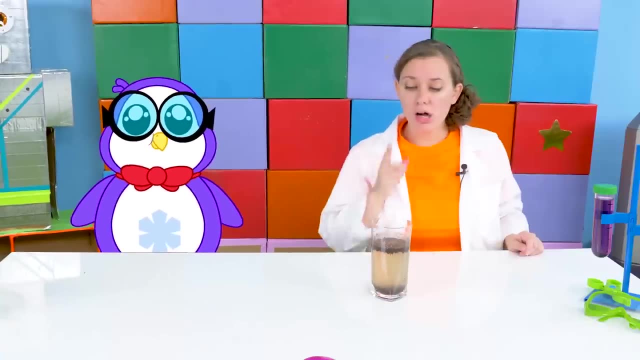 Well, Ryan sent us this glass of water, but it is really dirty, so I think we need to somehow clean it up. I think we should make a filter to get rid of the dirt. Oh, that is a great idea, But how are we going to make a filter? 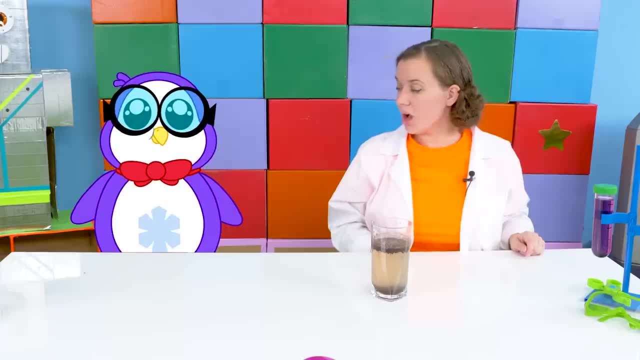 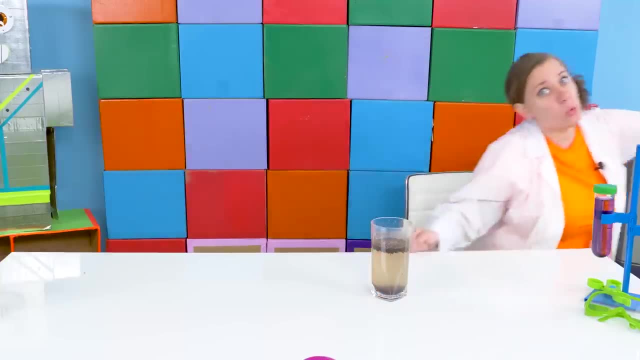 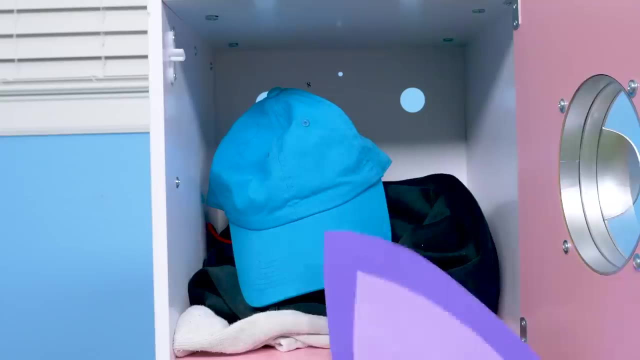 I think we can use everyday household items. Oh, I think I know some stuff that we could use- Me too. Let's get to it, Let's go. Hmm, Something to use as a filter, Maybe something in the dryer? Let's see. Oh, here we go, A sock. 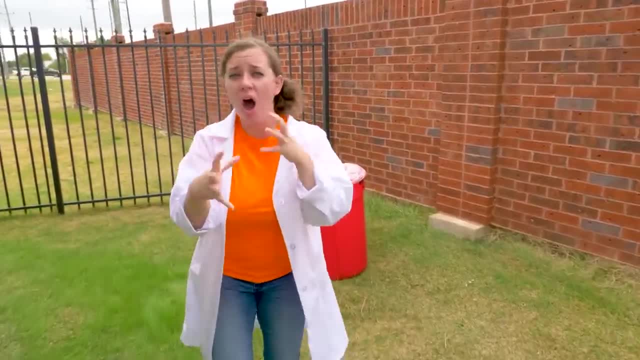 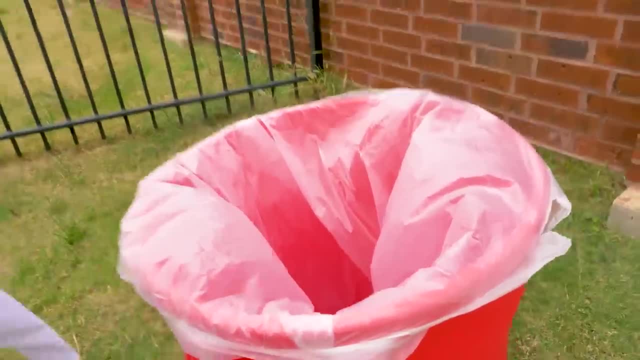 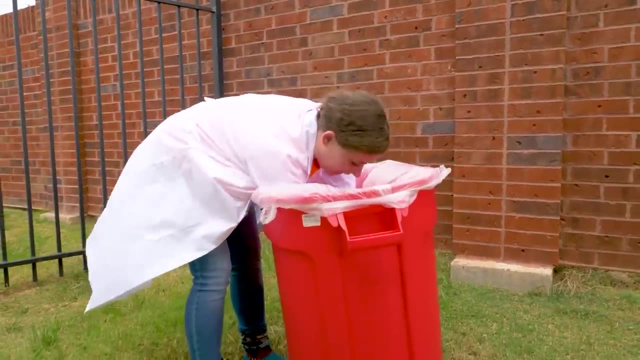 But I don't know what. Do you guys see anything? Of course There's probably something in here. Let's check. No, not that. Oh, no, not that. Oh, my goodness, This is perfect, It's going to work great. 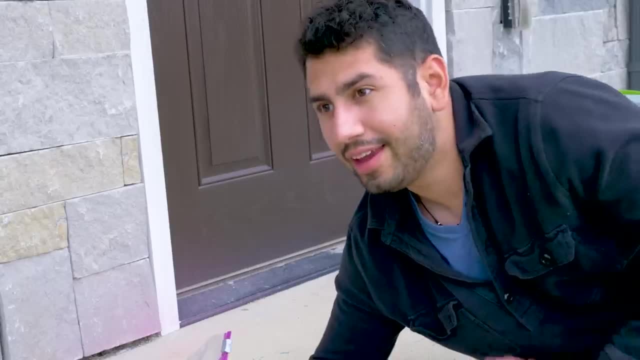 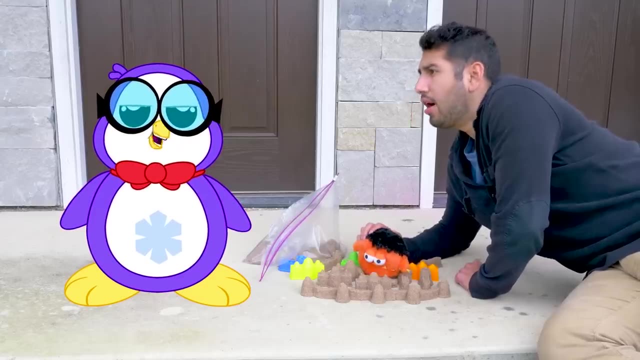 Oh hey, Daniel, Is that sand you're playing with? Oh hey, Peg. Yeah, I'm making some sand castles. Do you want to play with me? Uh no, I'm actually here doing a science experiment, but I could use the sand. 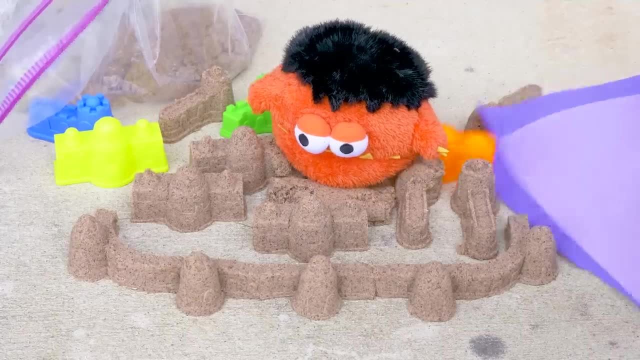 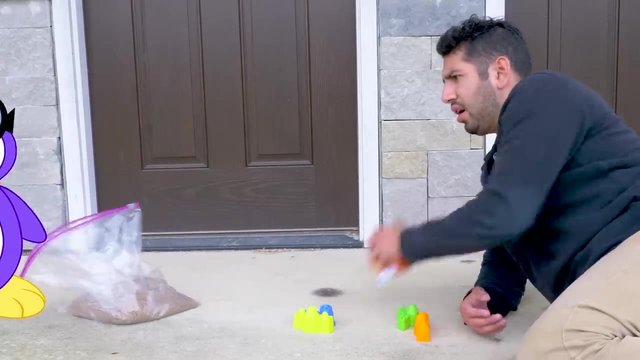 Yeah, of course Here, take some Gee. thanks, Daniel, Don't mind if I do. Thanks for your contribution to science. What? Oh, okay, Fine, I guess Take it all. I mean I wasn't using it or anything. 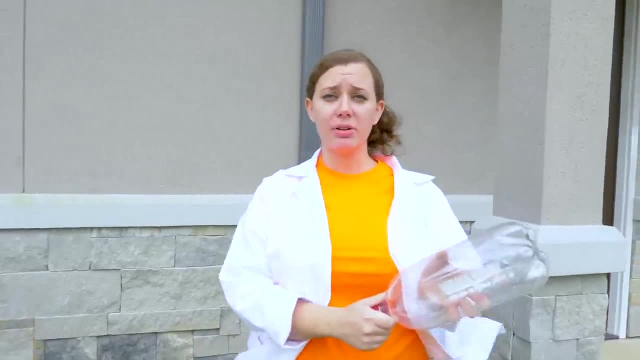 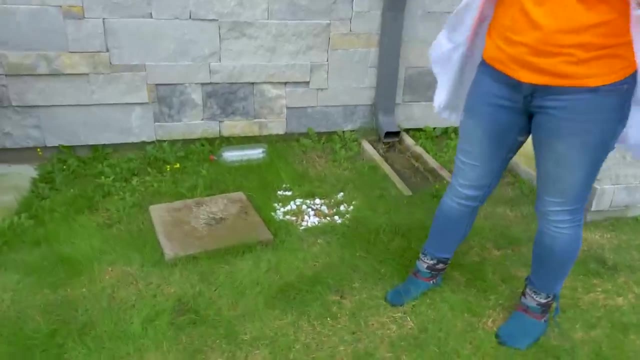 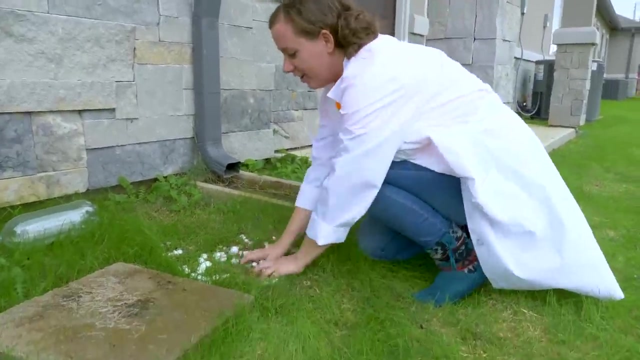 Hmm, So I got my bottle, but we need things to build the actual filter. So what could we use? What could we? I got it. We can use these rocks. They're perfect. There's so many of them, Man, this is going to work so good. 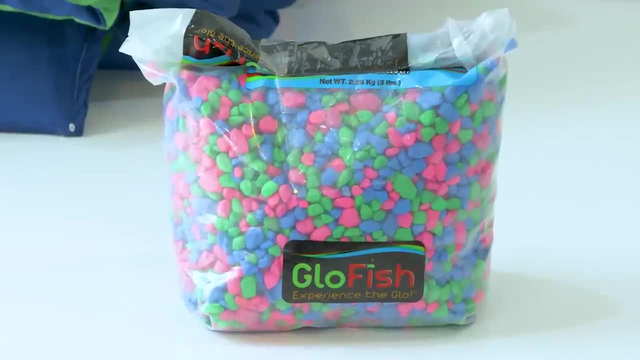 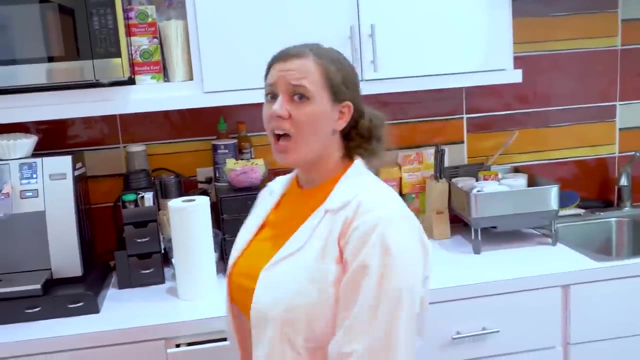 Ooh, a shiny bag of fish gravel. I can totally use this to help filter out the dirt too. Here we go, Hmm. Well, we're in the kitchen right now and there's got to be really good stuff that we can use as a filter. 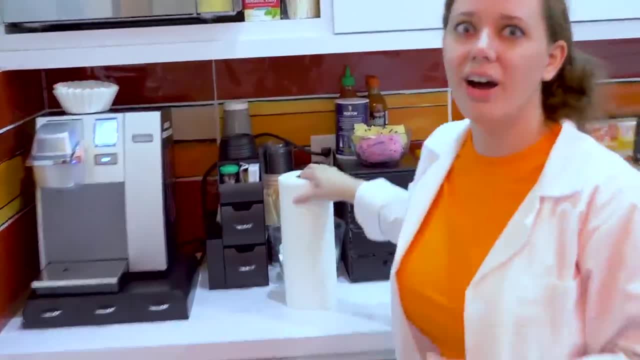 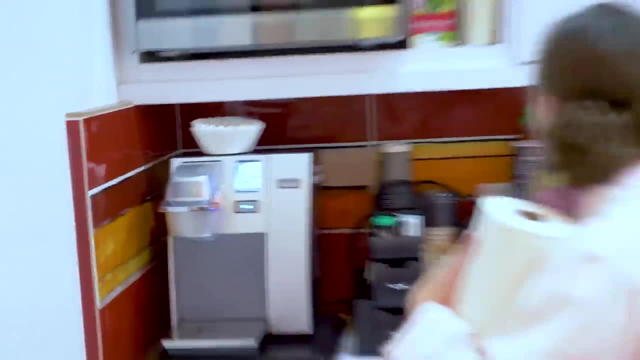 So let's see. Hmm, Of course, paper towels. That should work pretty good. I wonder if there's anything else. Um, no, Coffee filters. I think these items are great, but let's see what Peg's got. 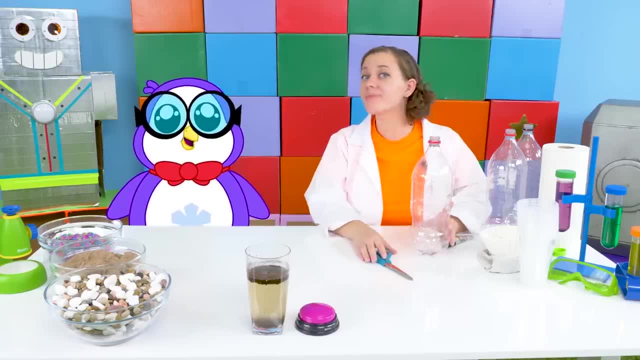 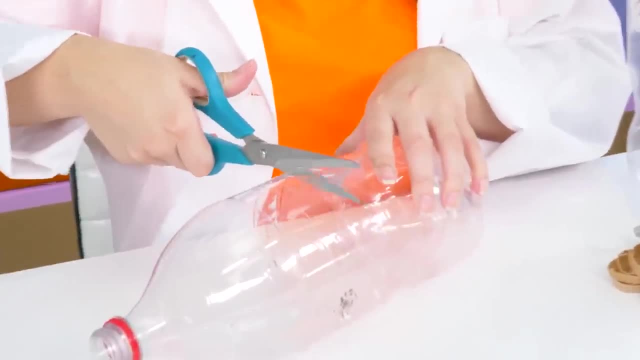 Woo, We gathered all of the needed materials and the tools. What do we do now? So the first thing we need to do is to make the outside of our container or our filter by cutting up this water bottle. Ooh, that's looking so good. 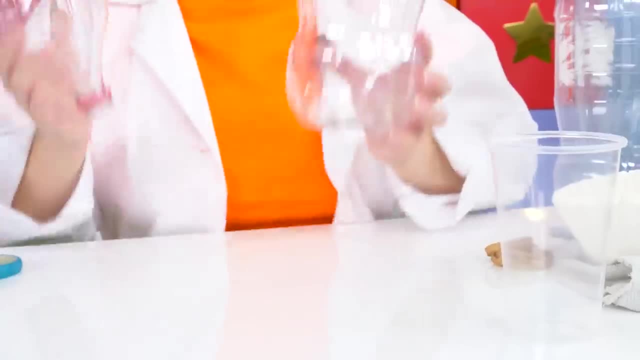 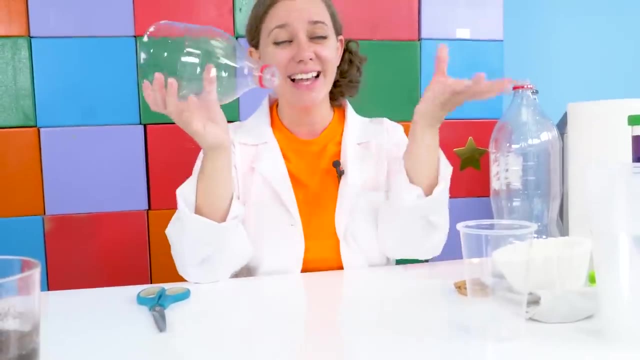 There we go. It's perfect. Now, the really cool part about using a bottle is we could use the bottom part to catch all of our water. but I found this cup here and I really like it because of how tall it is. 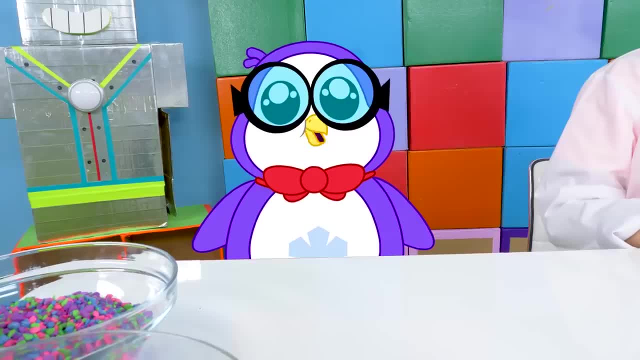 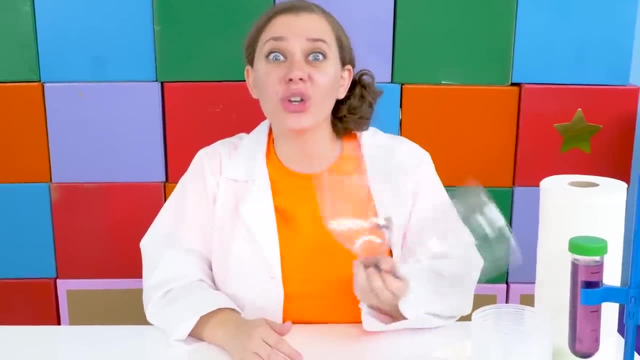 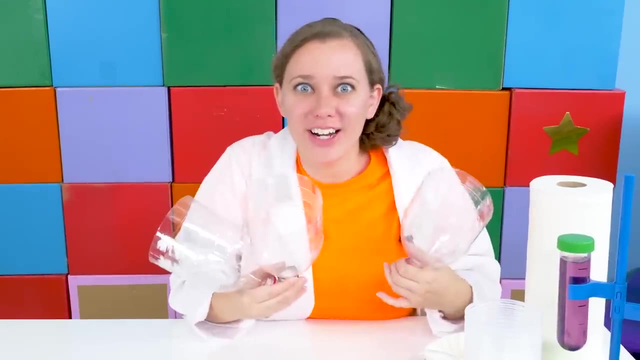 and I think we're going to be able to see our results really well in this. Ooh, I see Now that we've finished our first bottle. all we need is two and three bottles. That is perfect for our experiment. Let's get started. 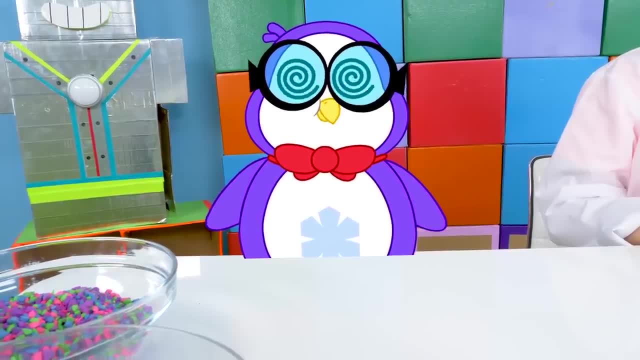 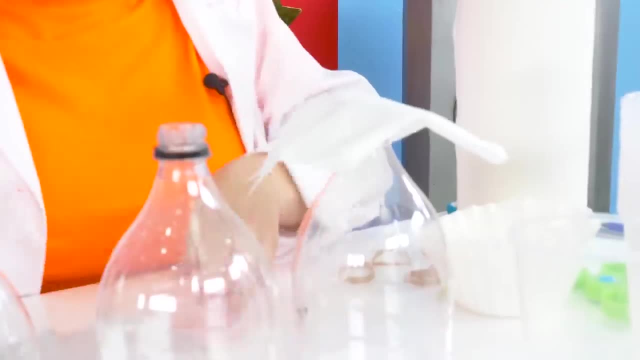 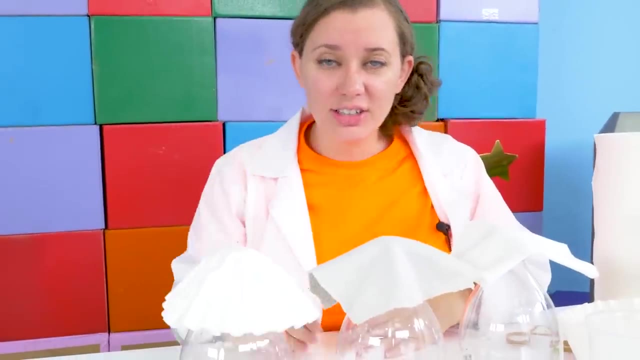 How'd you do that? I must be seeing things Alright. now we're going to start with our three different filter bases. So paper towels is our first one- Ugh, this dirty old sock. Is number two, And coffee filters is our third one. 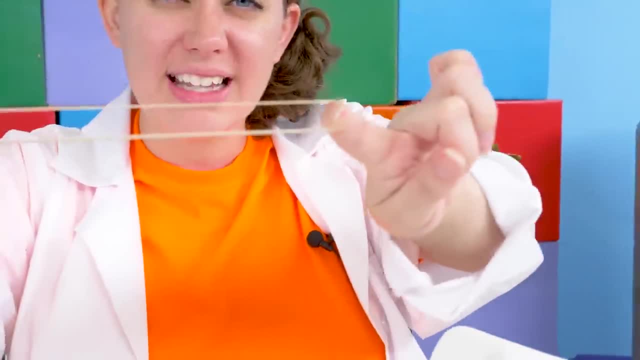 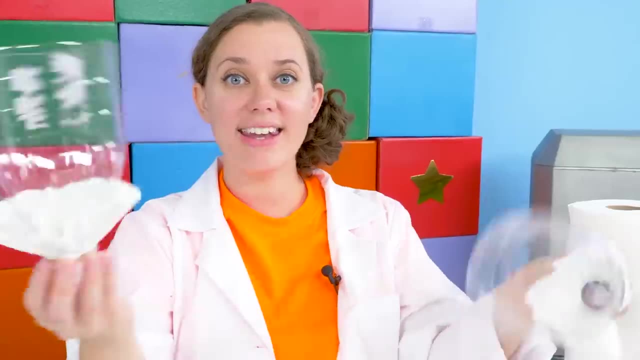 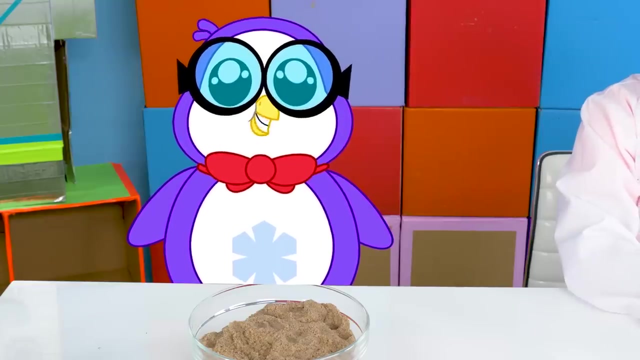 We can hold them into place with these really strong rubber bands. Okay, rubber bands One, Two, Three, Nice and secure. Hey, Peck, could you pass me the sand? One bowl of sand coming right up. Whoa, that looks like fun. 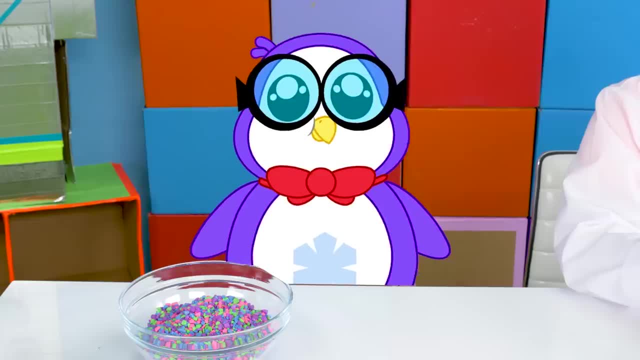 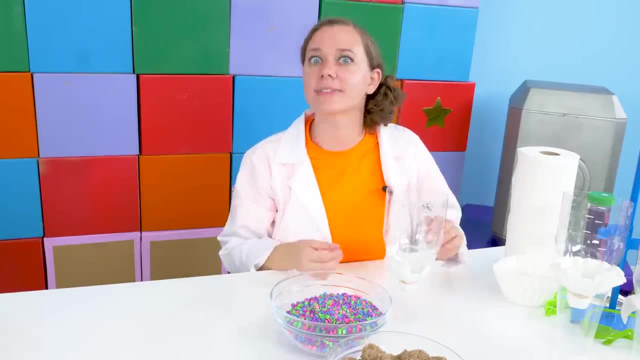 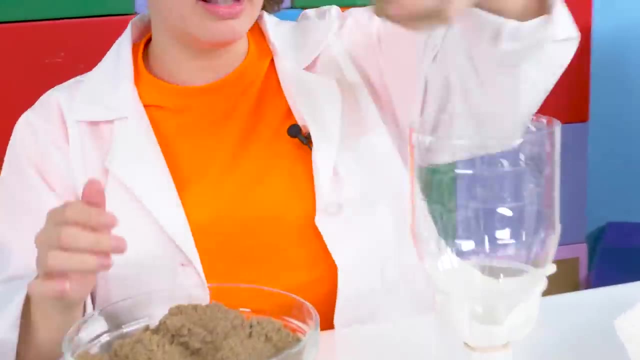 Next we need, Oh, gravel. Here's some gravelly gravel. Last thing that we need is rocks: Mm-hmm, big rocks, Uh yeah, Whoa, that's perfect, Alright, starting with the sand, Well, we have to make sure it goes all the way down to the bottom. so 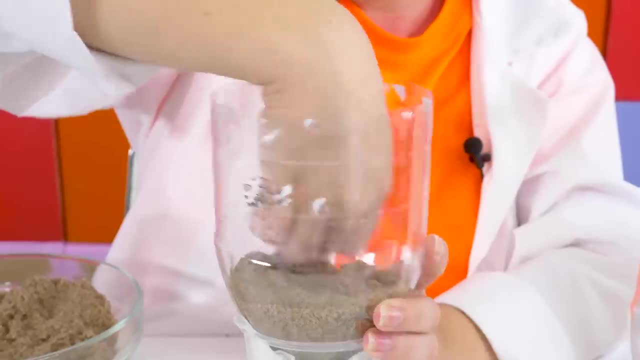 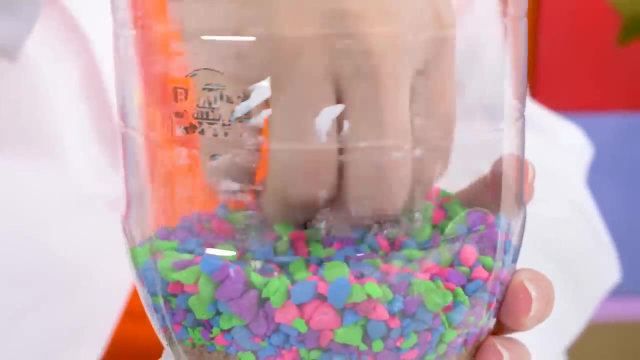 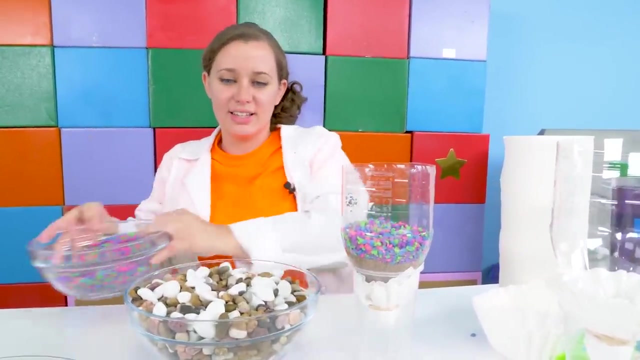 This kinetic sand is nice. It doesn't get messy. Next up is the gravel. This is going to be so pretty. I love the colors. I think that looks pretty good. So now we need these big, heavy rocks. Looking good. Hey, can I borrow one of those pebbles later? 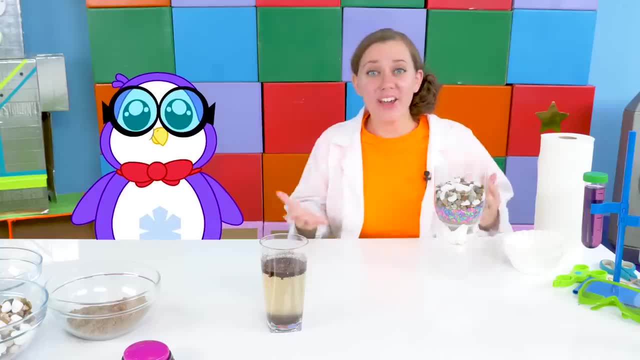 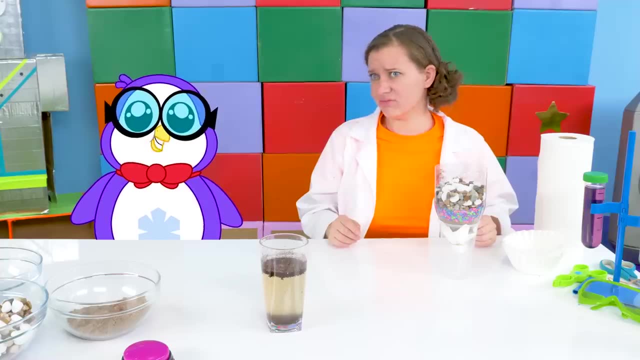 There you go. That looks pretty good Now that we have our first one built all the way. we just have to do the same for two and three. Oh, I can use my special blaster to get the job done, Pew, Oh. 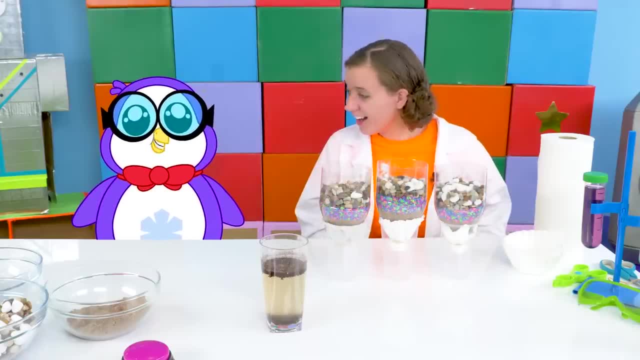 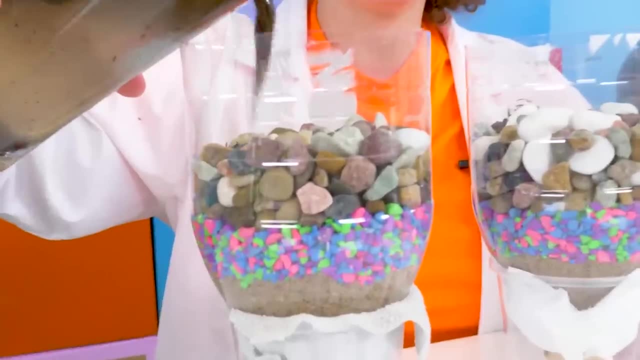 Whoa, that is incredible. Aw shucks, It was nothing. Okay, here's a moment of truth. Let's see if our filters work. Ooh, I can see the water filling up and the little pieces of dirt swimming around like fish. 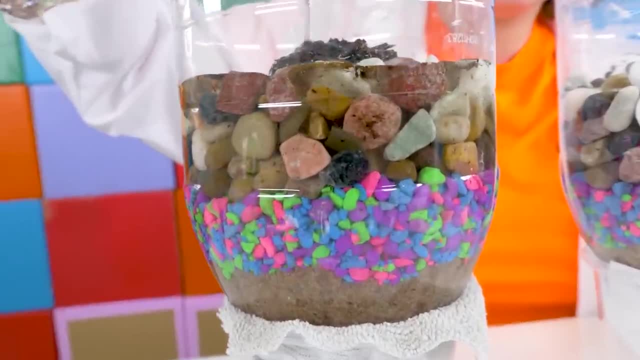 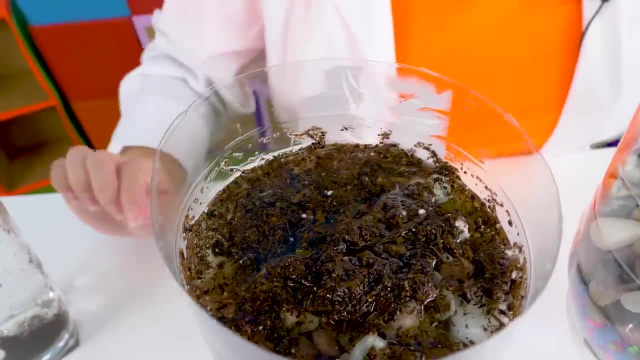 I'm getting a little hungry now. We're already starting to get some water coming out. Whoa, look at that. It looks like a lot of the dirt is getting caught by the sand. The dirt is getting caught by these rocks and maybe some of the smaller dirt by these smaller rocks. 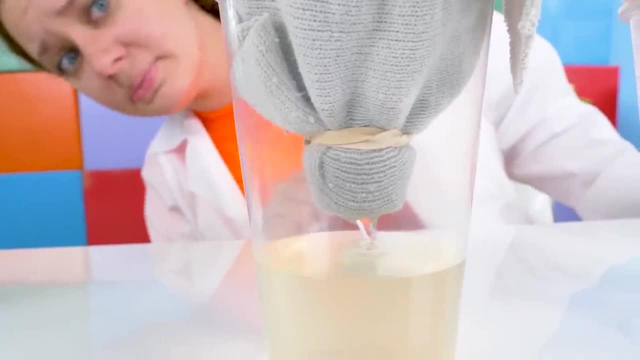 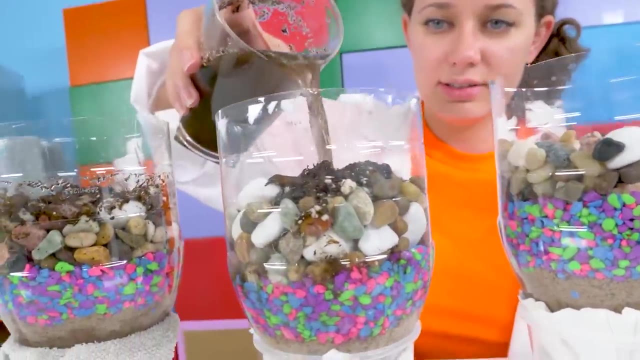 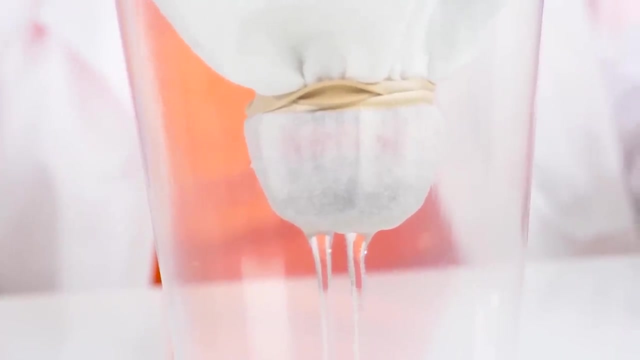 The sand looks like it's doing a lot of work too. Four times speed, Whoa. All right, let's see how the paper towel does Whoa. That rubber band sure is doing its job. And the last one is the coffee filter. 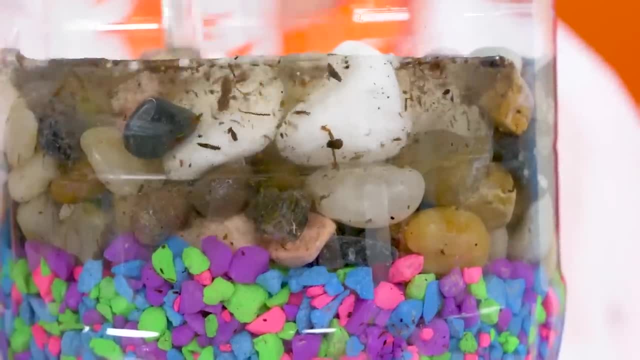 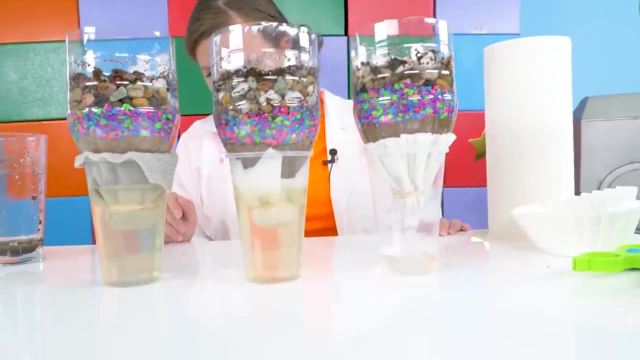 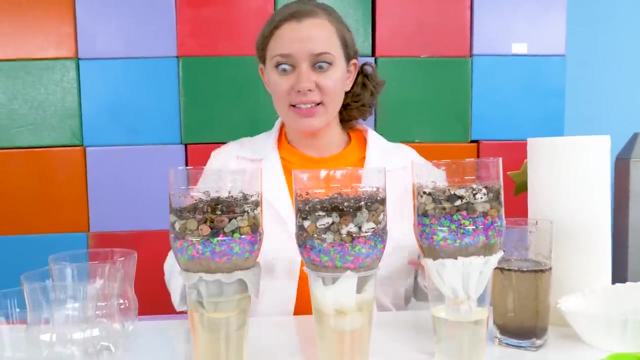 I mean, it is a filter. It's a coffee filter on the end of a filter, Whoa. So this one looks like it's already coming out more clear than the other two. Brilliant deduction, Bri. Now that we have all of our water filtered, let's take a look. 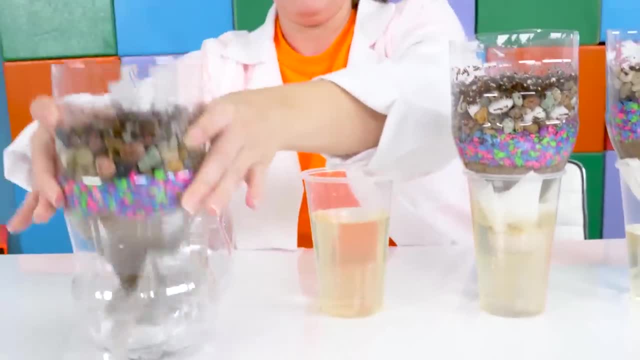 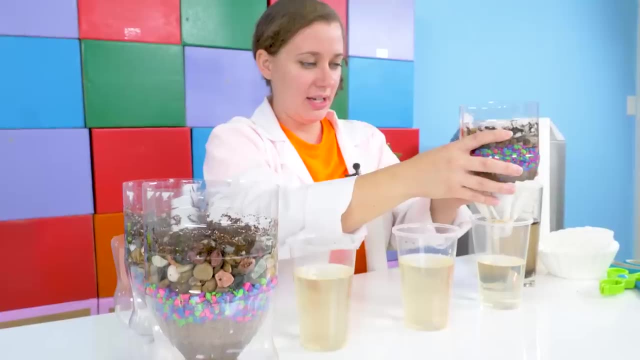 Let's compare them. Okay, so we're just going to take these guys out and put them in here. Oh gosh, be careful. Ooh, There we go. And last but not least, the coffee filter. Yay. 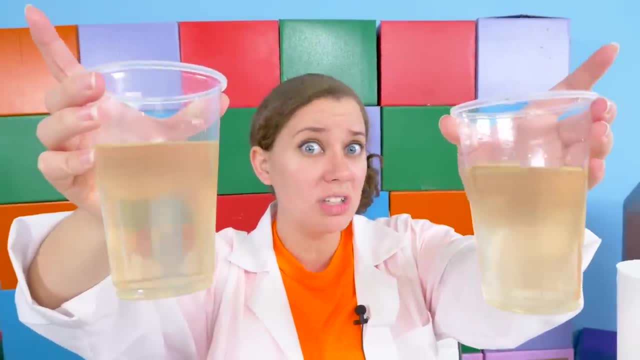 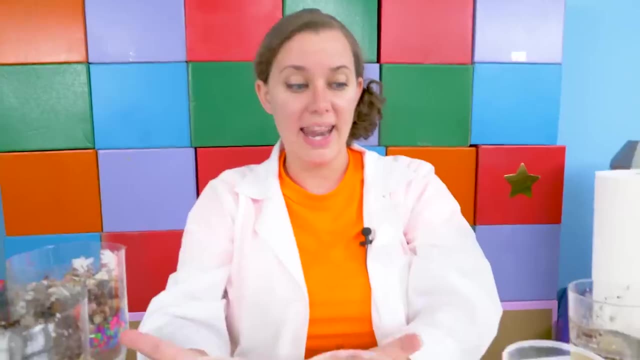 Well, these two, I don't think they did as well. It worked a lot. There's obviously no dirt in there, but they look pretty cloudy and I can't really see through them that. well, Now the coffee filter: Whoa. 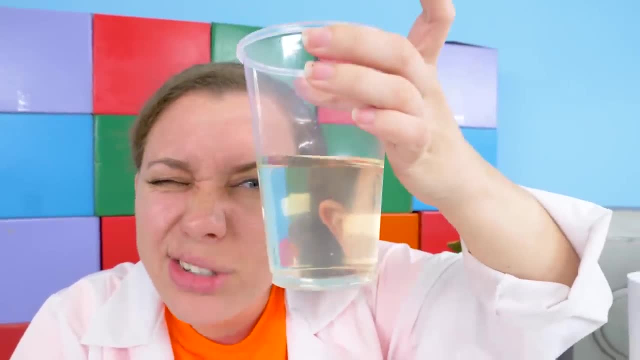 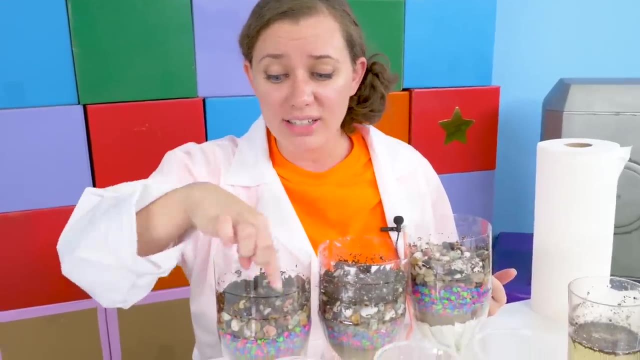 That is so clear. Look at that, I can see straight through it. It's time to review the results for Ryan. Okay, so I think the results show us that the rocks and the gravel and the sand do a really good job of getting all the dirt out. 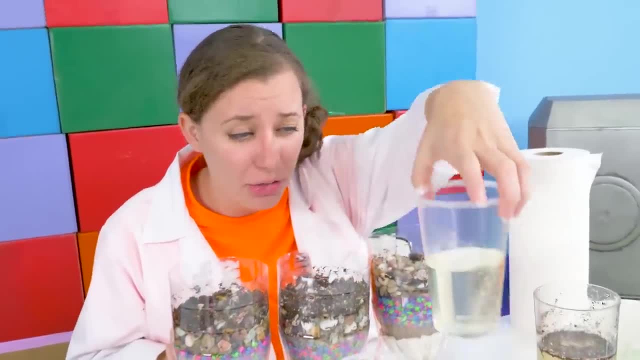 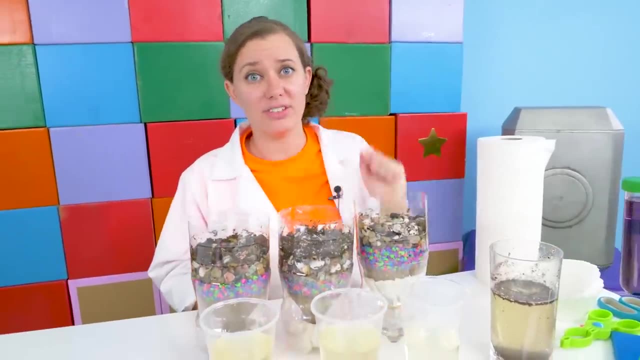 But the coffee filter isn't. The coffee filter is the only one that can get all those little teeny tiny parts out, which makes it clear like that. I think it's safe to say the coffee filter definitely did the best, But it does look better.